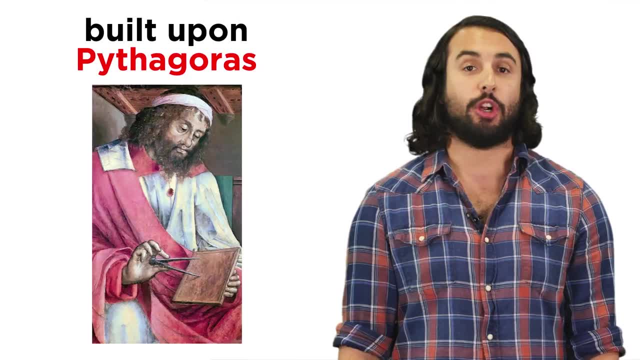 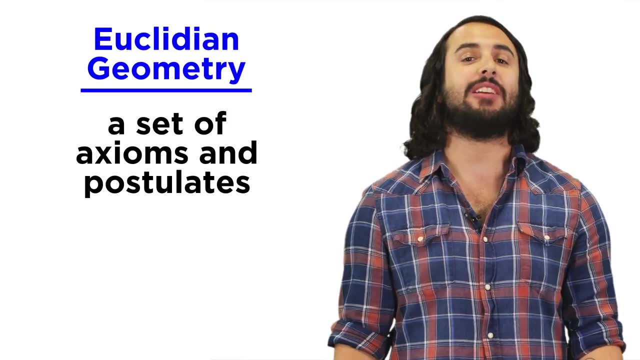 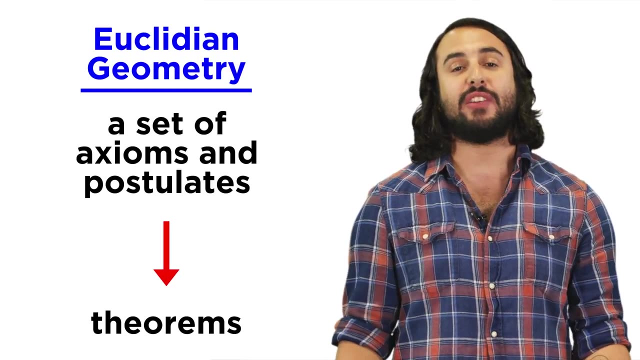 Euclid, to whom it is attributed. His work, which built upon the work of earlier mathematicians like Pythagoras, describes a set of axioms and postulates from which a variety of theorems can be derived. Let's learn about the physical constructs that these axioms describe, so that we can. 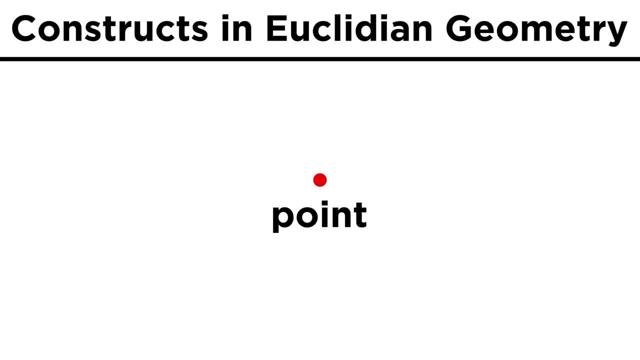 learn about all the math we can do with them. First we look at a point. This is nothing more than a location in space. It is zero-dimensional. Zero-dimensional meaning that it has no dimensions of any kind. We represent points with little dots and some capital letter, making sure to realize that. 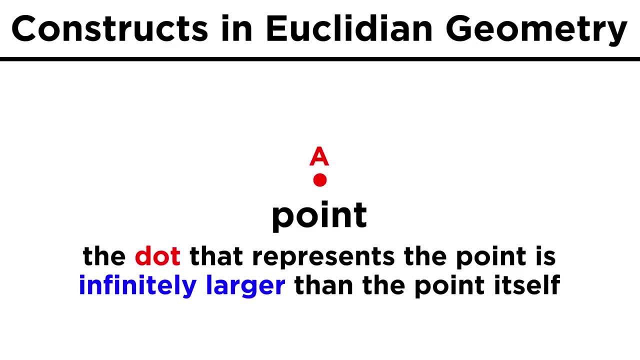 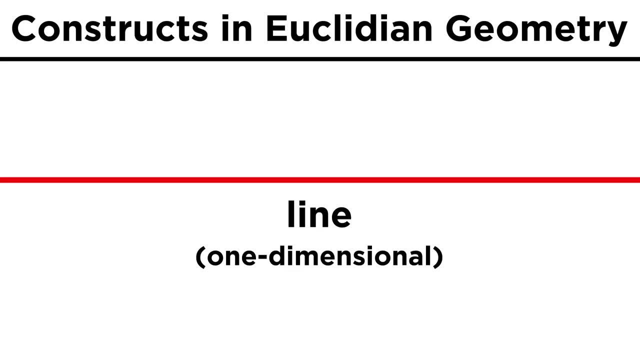 the dot we draw is infinitely larger than the point it is meant to represent. From here we can construct a one-dimensional object by stringing an infinite number of points along a particular dimension. This object is called a line. Points and lines are familiar to us from algebra. but now let's examine a two-dimensional. 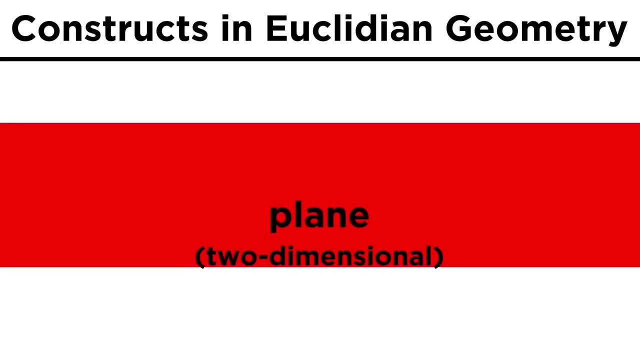 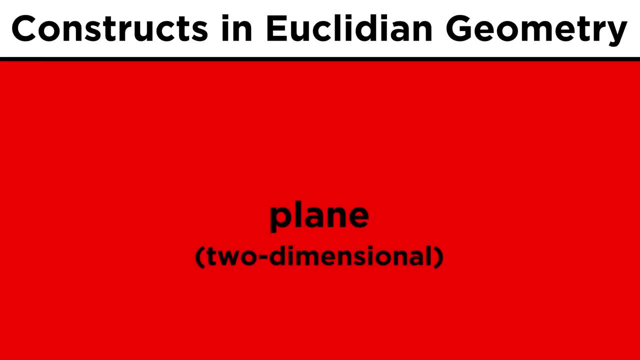 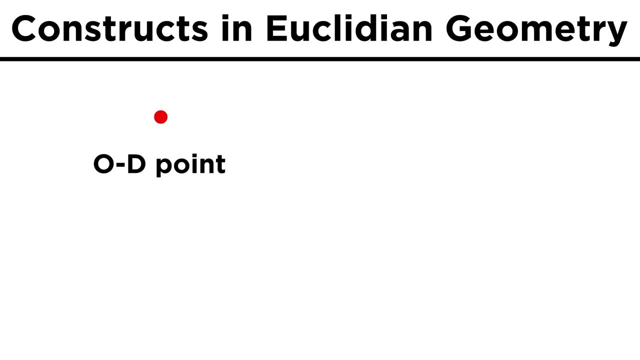 object. This can be achieved by stringing an infinite number of lines along a dimension perpendicular to the line. This is called a plane, And then, if we string an infinite number of planes in either direction, we get three-dimensional space: Point, line, plane space. 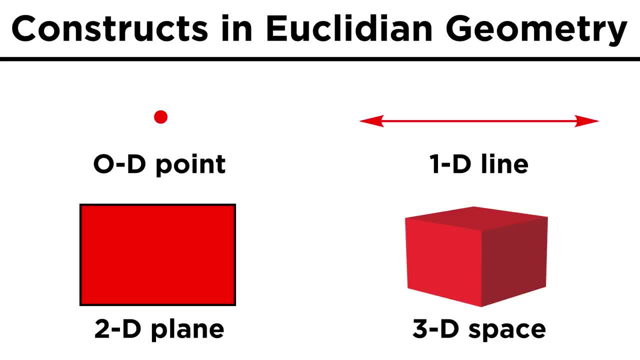 Zero one, two and three dimensions. Point line plane space Zero one, two and three dimensions. Point line plane space Zero one, two and three dimensions. Another linearity we can identify is that a point is just a point, but any two points. 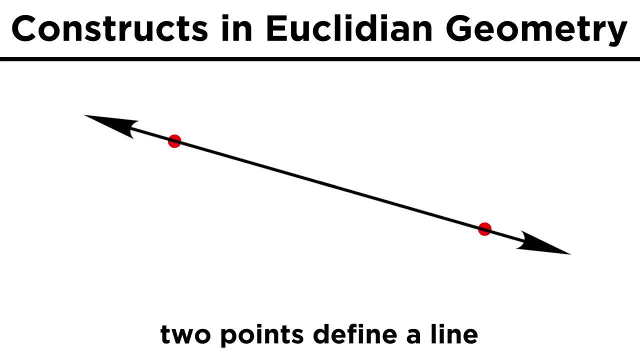 can define a line, since there is only one line that contains both of these points. Extrapolating further any three points that aren't all collinear can define a plane, since there is only one plane that contains all three of these points. 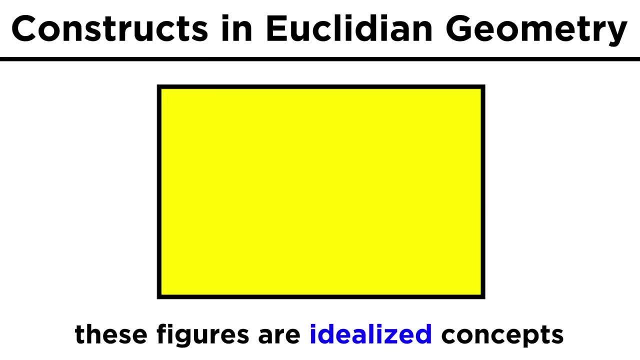 We should mention that these figures are idealized concepts. We can never create a plane. We can never create a plane that is infinitely thin so as to legitimately consist of only two spatial dimensions. Even a piece of paper has some thickness, even if it's hard to see with the human